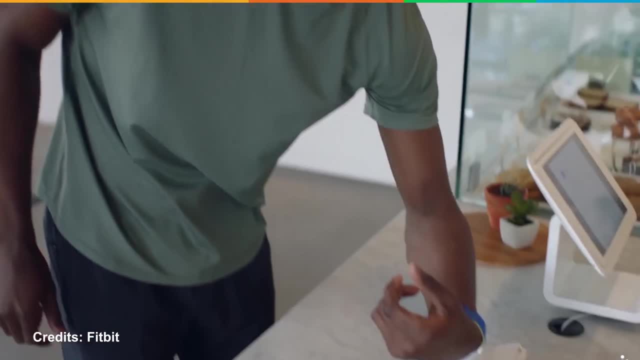 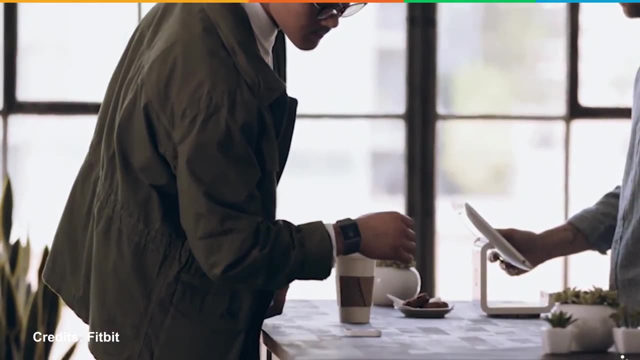 The smart money transfer technology can reduce the burden of mobile money transfer. When you're on the go, you could easily step into a store, purchase the goods and pay hassle-free. After every successful transaction, the balance is updated immediately to avoid any uncertainty. 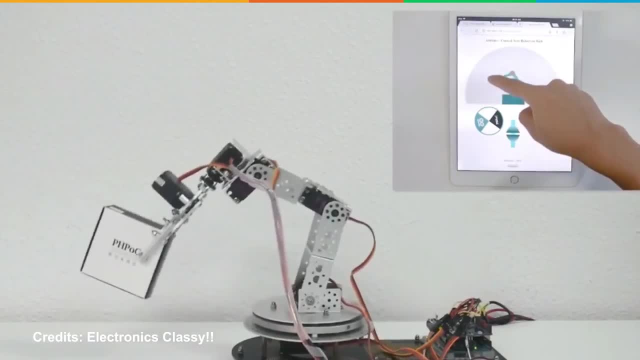 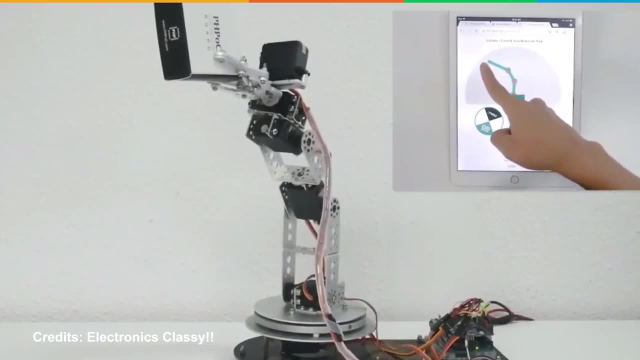 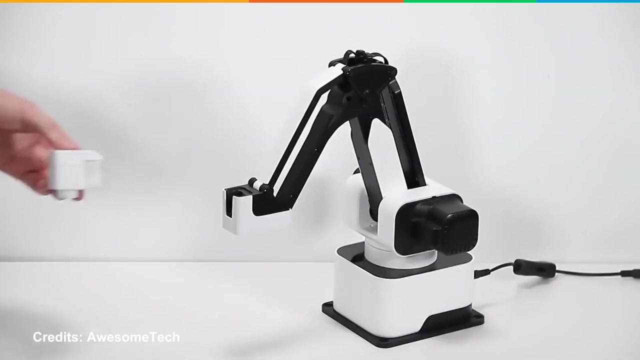 3. IoT-based Smart Arm. This project includes the creation of a robotic arm which can pick and place things from one place to another. To control this action, the robotic arm can be moved using specific commands. Some advanced arms allow the user to change the end effect of the arm. 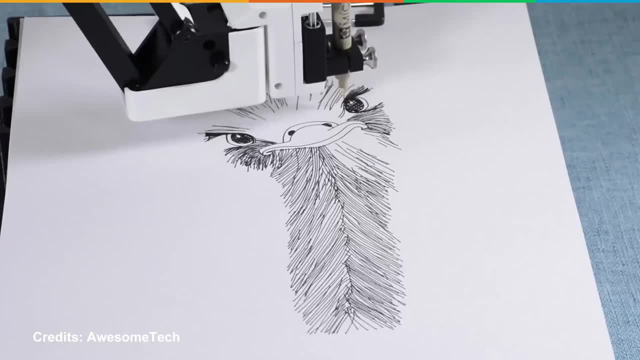 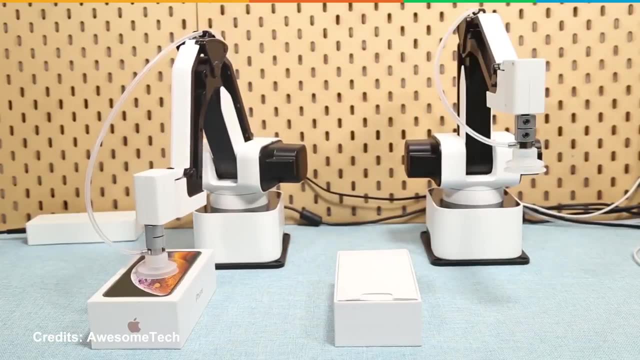 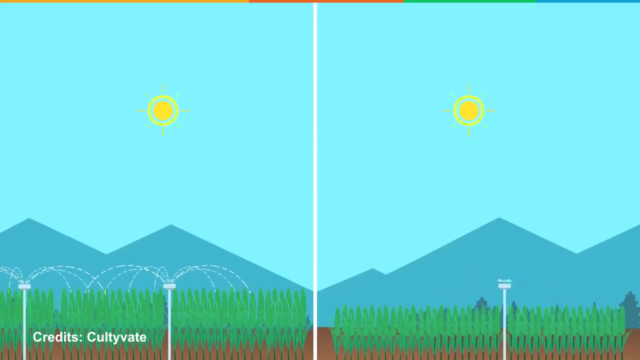 to perform various different actions. It can be used to make art, print 3D images and build production lines. It can also be used to perform your day-to-day chores. 4. Smart Irrigation. With change in climate and recurrent water crisis, farmers suffer a great deal with growing crops. 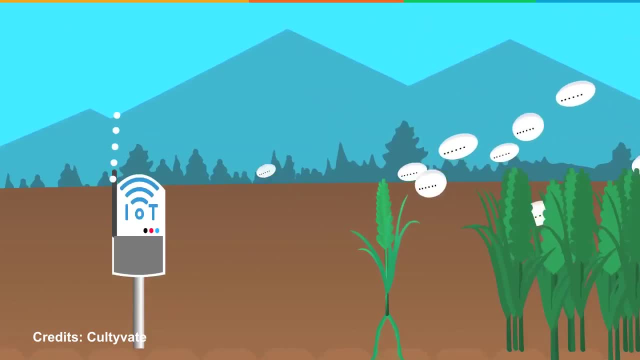 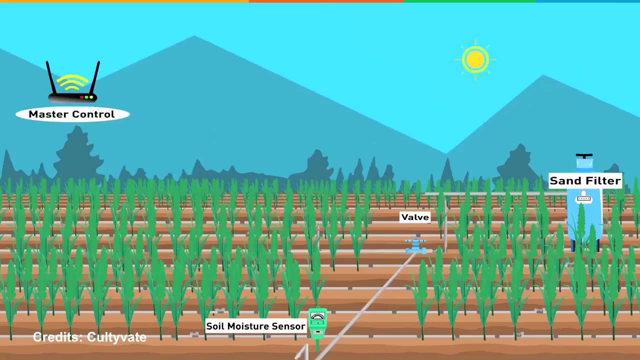 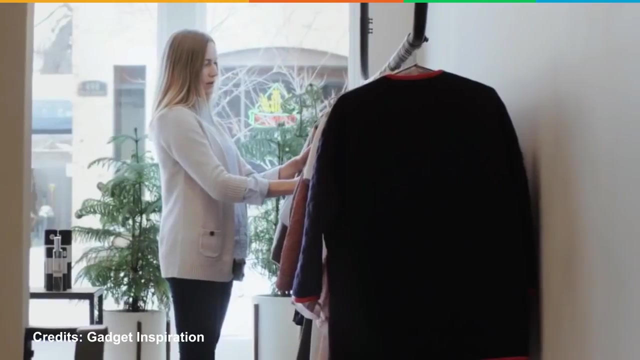 Smart irrigation puts an end to this ordeal. This system comes with a moisture sensor that checks the soil for its water content. When the soil moisture drops below a certain value, the The system triggers the water supply. At number 5, we have Smart Door. 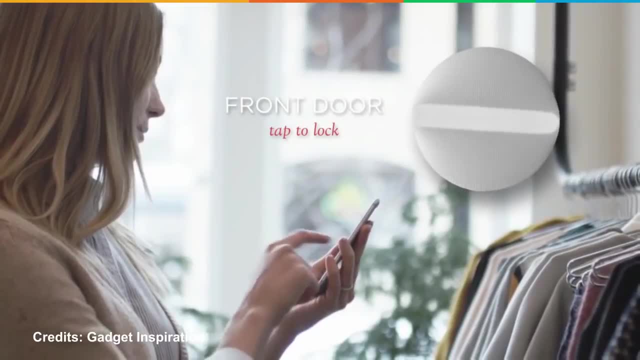 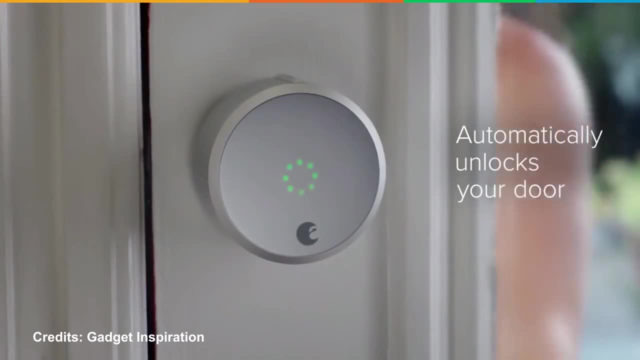 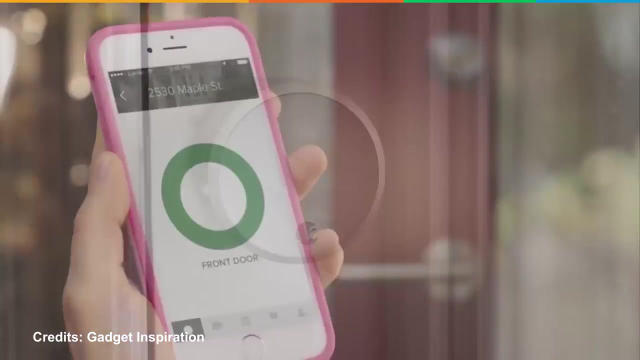 As the name suggests, this project aims at creating smart doors that control the entry and exit of humans. These doors open and close automatically when you pass by The door- can also be controlled remotely. You could unlock the door for a friend by tapping an icon on your smartphone. 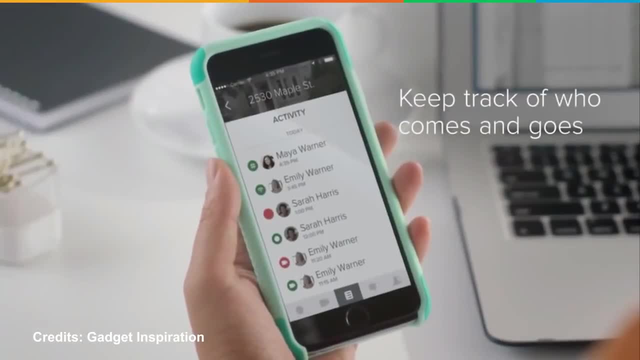 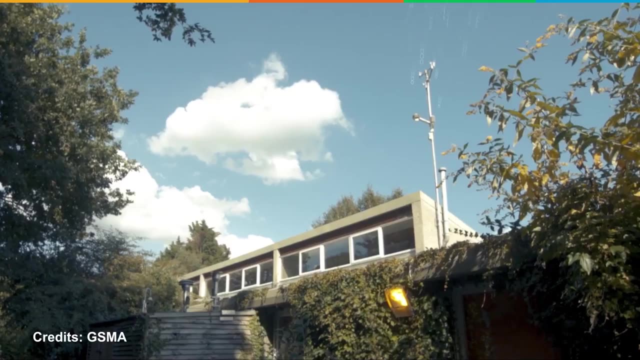 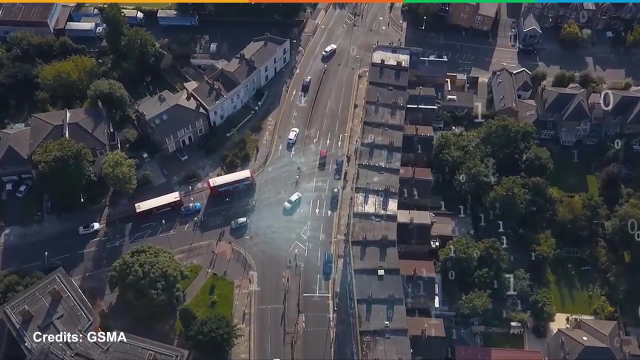 Once they exit, you're immediately notified. The owner can also choose who has the access to the door. At number 6, we have Air Monitoring System. Now air monitoring has become crucial for the environment, and what better way to do it than incorporating IoT. 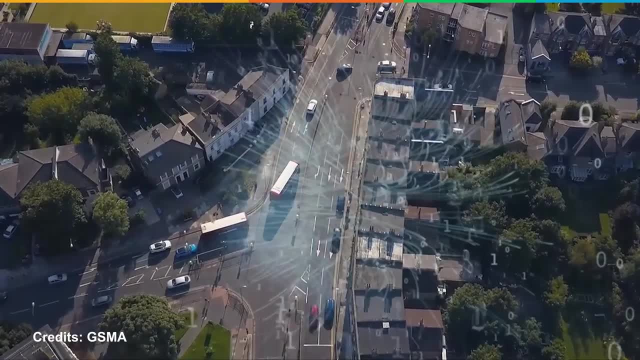 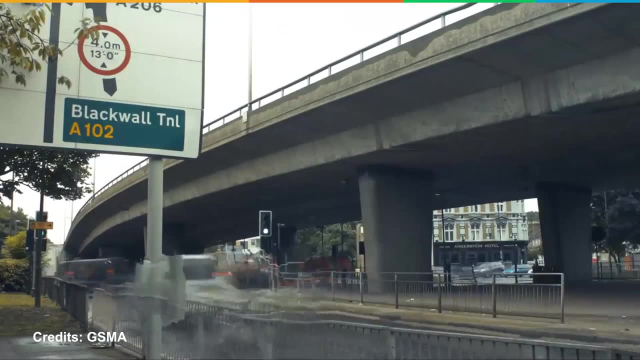 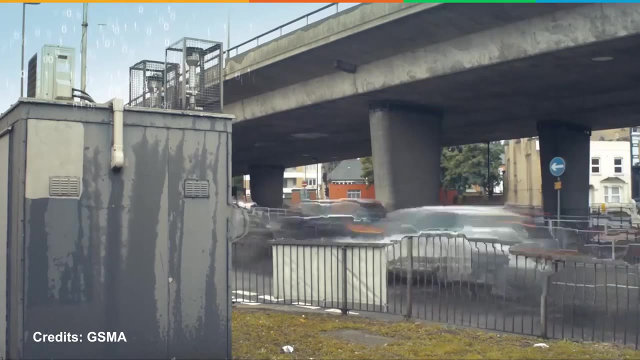 The IoT system uses air sensors to sense the presence of harmful gases or compounds in the air. The data collected can be used by the local authorities to make a detailed analysis. Necessary actions can also be taken To ensure that the air quality levels don't reach an extreme low, especially in areas 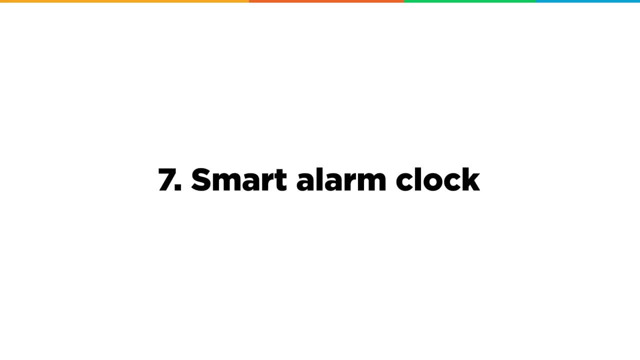 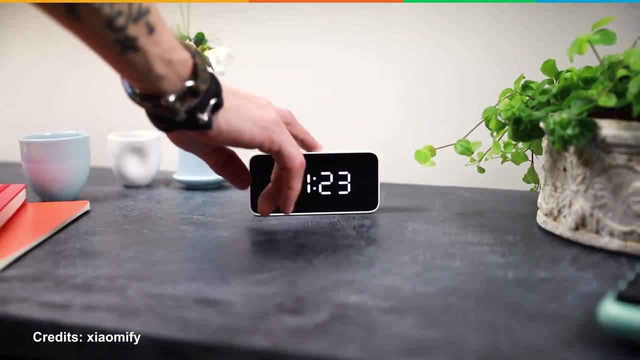 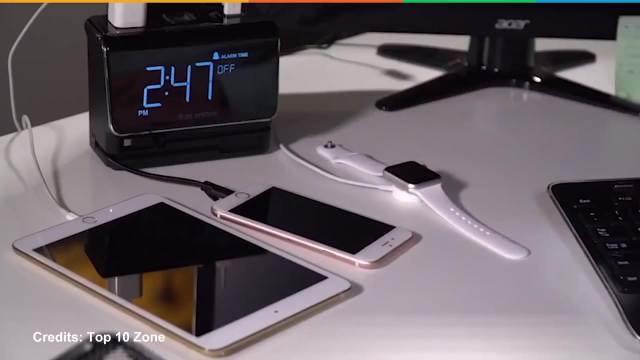 with hospitals and schools. Moving on to number 7, we have Smart Alarm Clock. Now there are many variations of a smart alarm clock, But the alarm we are talking about is a self-setting alarm. This smart alarm clock uses your Google Calendar to check your appointments, to set the alarm. 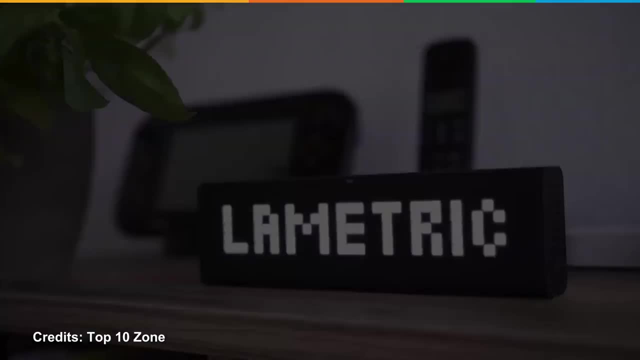 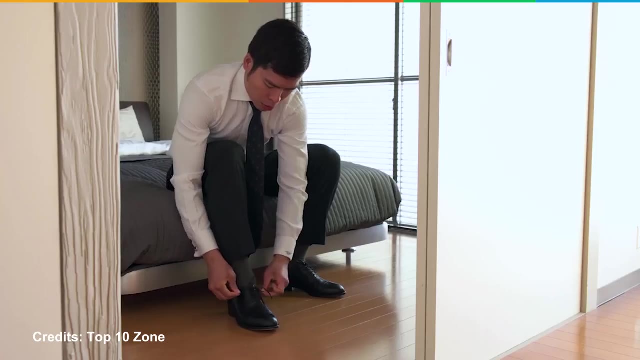 It can also procure data from GPS. This smart alarm clock uses your Google Calendar to check your appointments to set the alarm. It can also procure data from GPS about your ETA to a particular place and consider the weather to automatically adjust your wake time. All of this is just making life more easier. 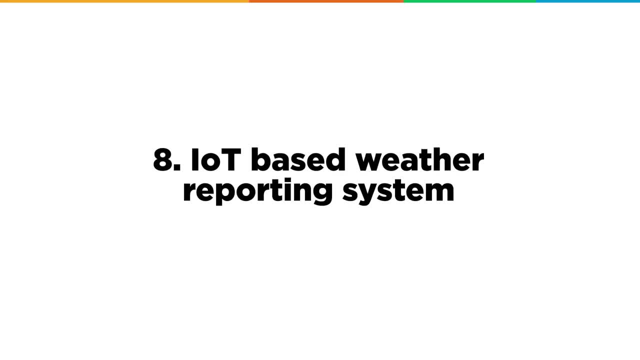 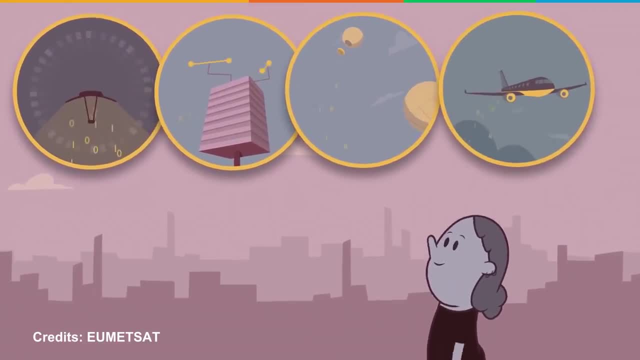 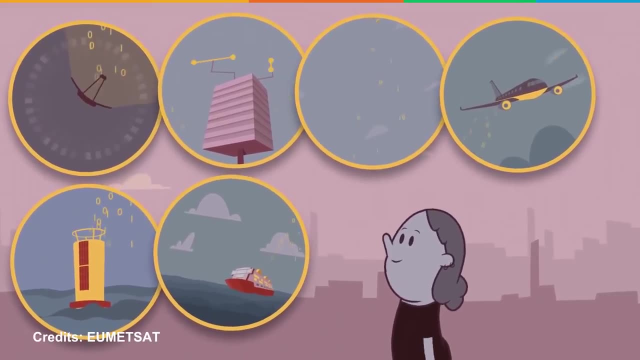 Moving on at number 8, we have IoT-based Weather Reporting System. Now the system deals with monitoring weather and climate changes like humidity, temperature, moisture, wind speed, UV radiation, light intensity and even carbon monoxide levels in the air, using multiple sensors. 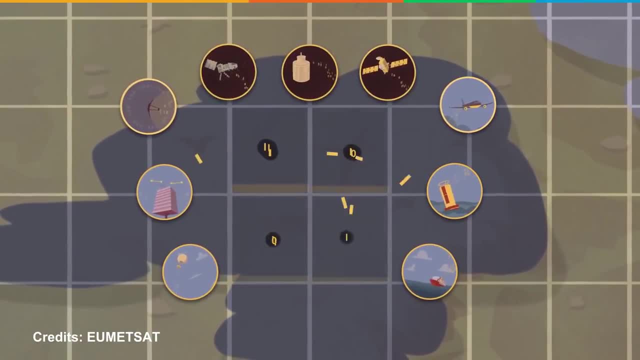 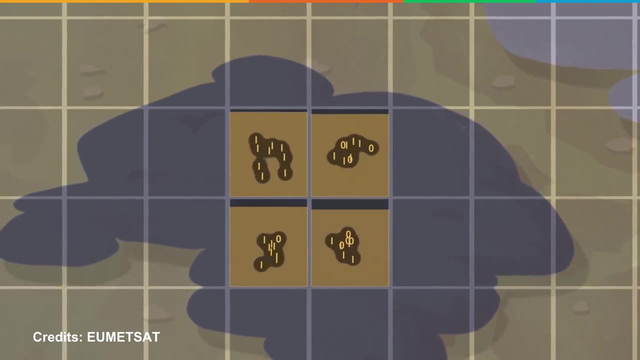 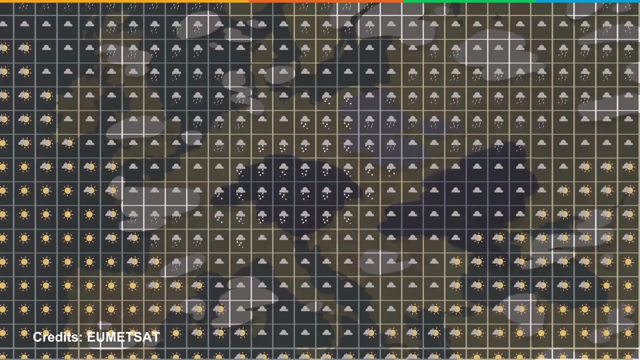 These installed sensors send data to the web page that is plotted as graphical statistics. The project even consists of an application that sends notifications as an effective alert to warn people about sudden and drastic weather changes. So when you're heading out, the app could easily tell you what the weather will be like. 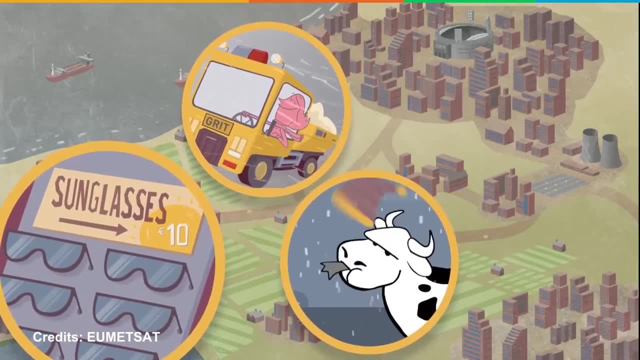 and suggest carrying an umbrella or perhaps a sunblock. At number 8, we have Smart Alarm Clock. This smart alarm clock uses your Google Calendar to check your wake time and consider the weather changes. At number 9, we have Smart Wheelchair. 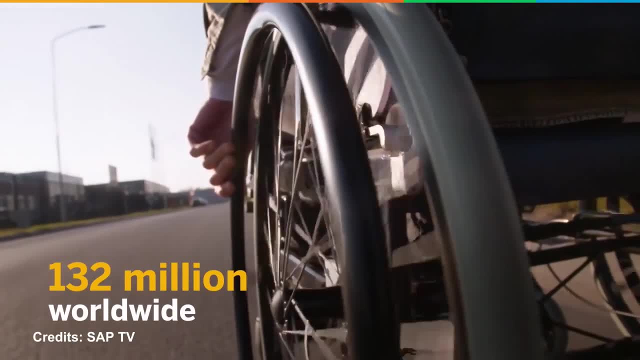 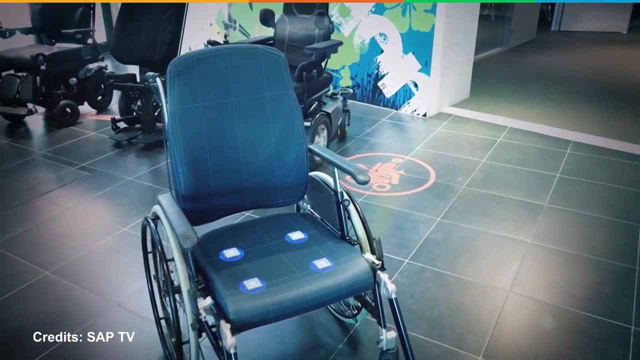 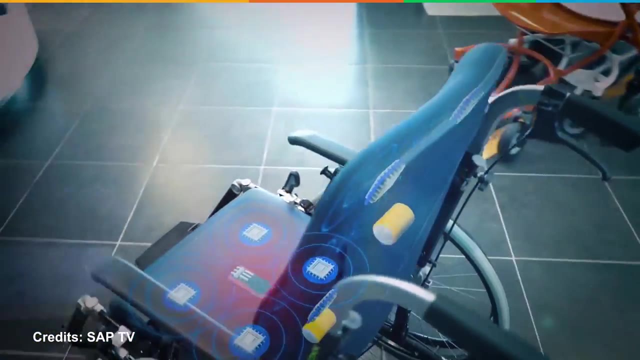 There are over 132 million wheelchair users across the globe. Smart Wheelchairs is an excellent innovation. Typically, it comes with built-in sensors on the seats that collect data every second. The data provides insight into the seating behavior of the patient and the energy required. 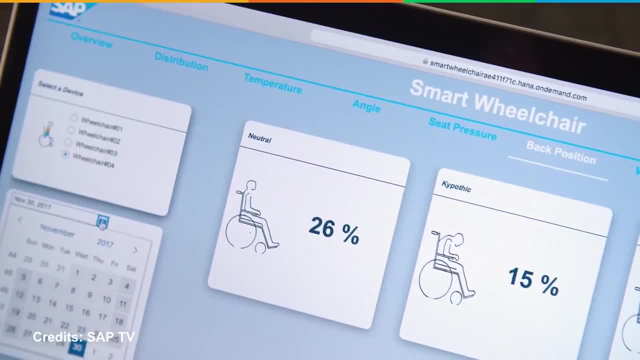 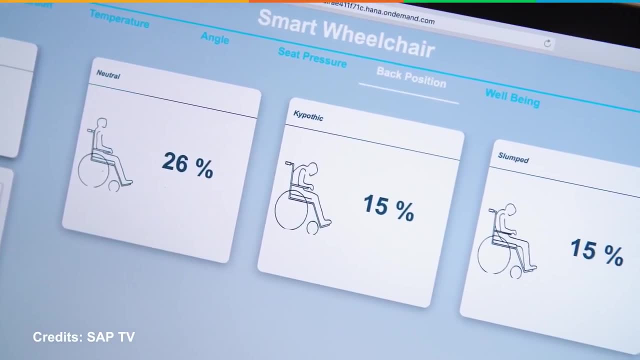 to maintain the posture. Other variations of Smart Wheelchairs include the Smart Wheelchair. It has a combination of two: Fault Detection and Smart Wheelchairs. These features allow people to monitor the patient from a remote location. And finally, at number 10, we have Smart Street Light system.